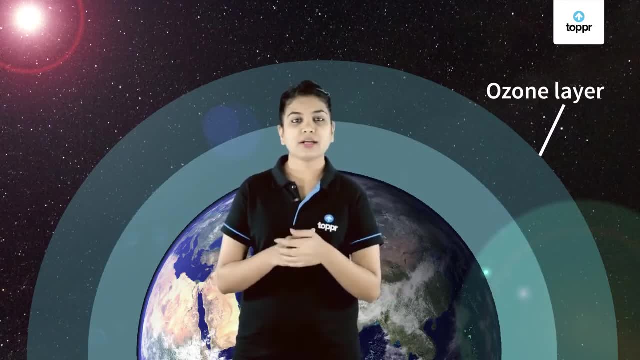 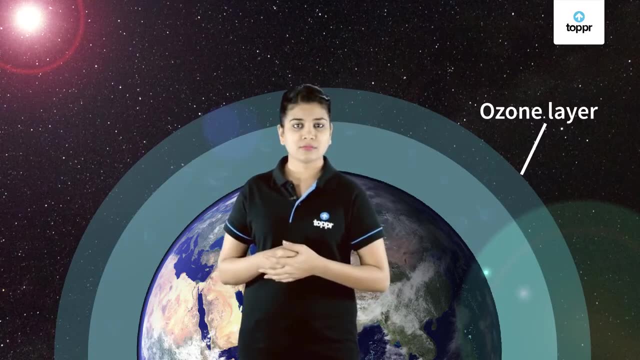 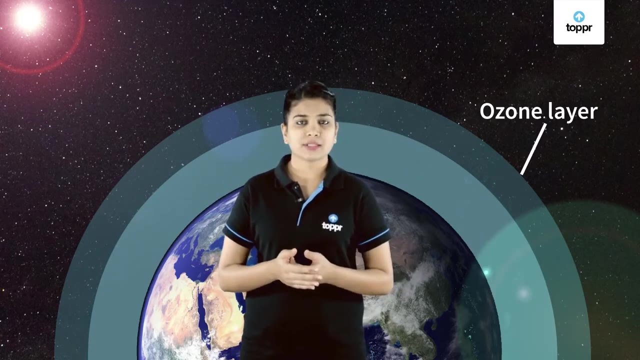 recently it has been found that this ozone layer it is depleting, which means it is getting reduced. But how is it happening? The various man-made compounds, like CFCs, which are close to the Earth's surface, They contain chlorofluorocarbon, They contain 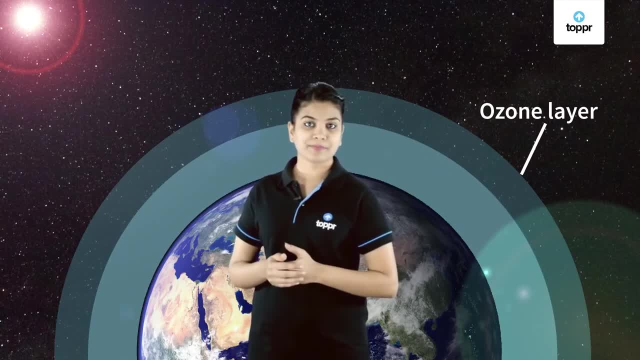 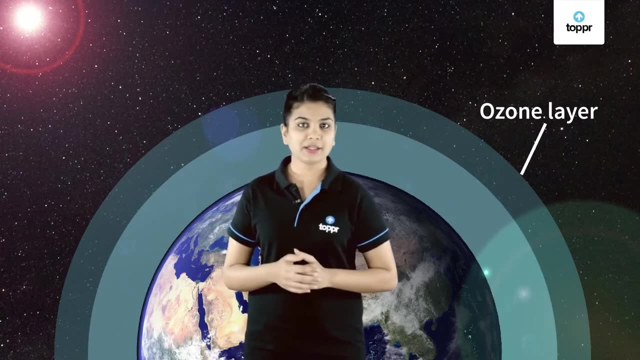 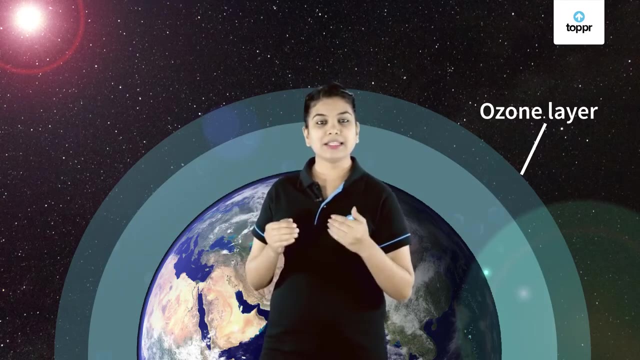 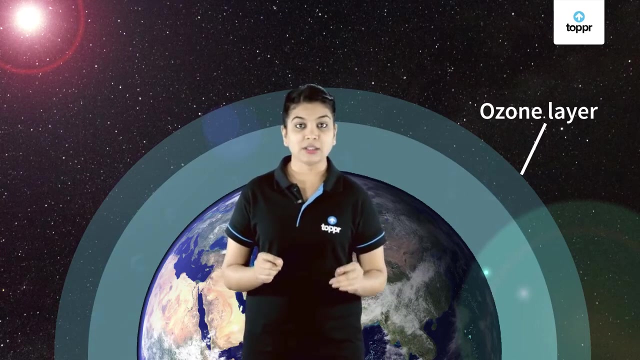 chlorine as well as fluorine in them. They are found to be very, very stable. They persist in the atmosphere and they cannot be degraded by any biological process. So when they reach the atmosphere they react with ozone. Their reaction now causes the reduction in the 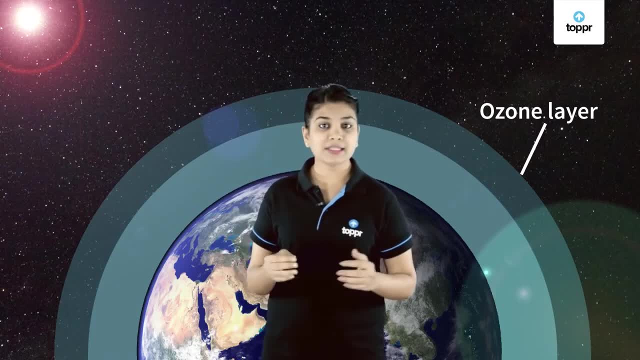 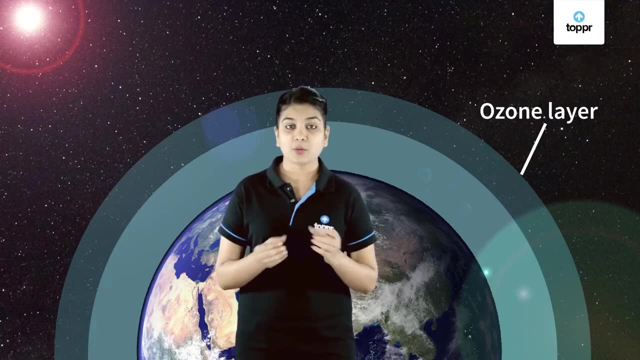 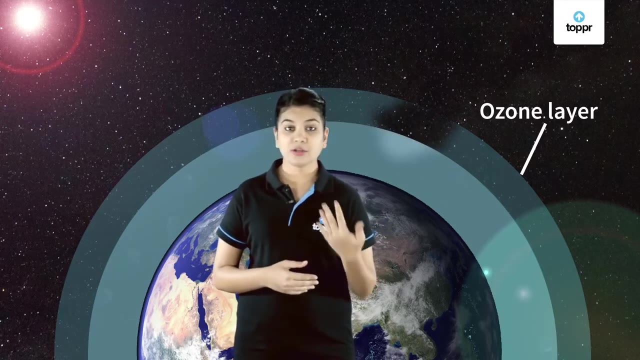 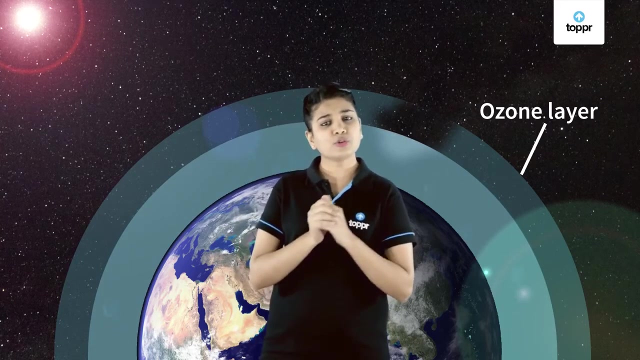 ozone layer. It is a very serious issue, In fact. this ozone, it has been found to reduced up to that extent where a hole has been found in the region of Antarctica. We cannot even imagine the consequences if this ozone layer further reduces. So we should do. 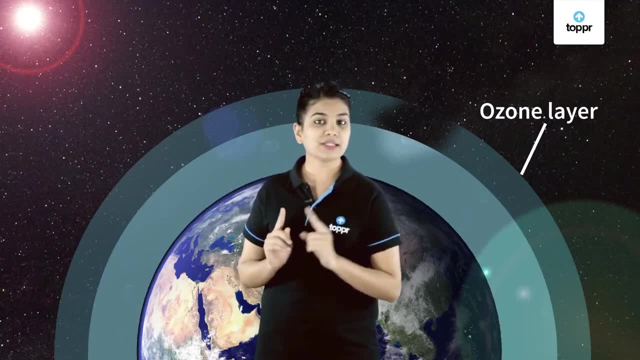 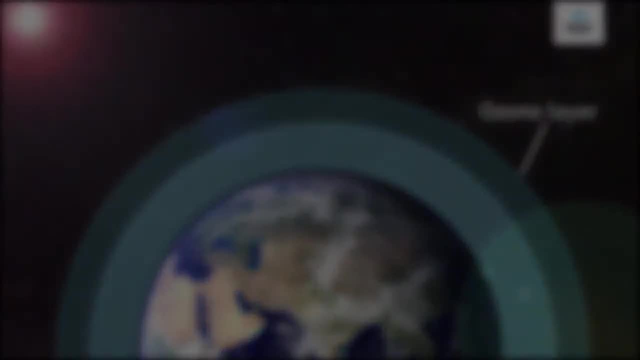 something to avoid the further depletion of this ozone layer. So we have learned that CFCs they cause the depletion. right Now, these CFCs, let's see what is the chemical reaction they cause. So firstly, we'll see the excessive use of 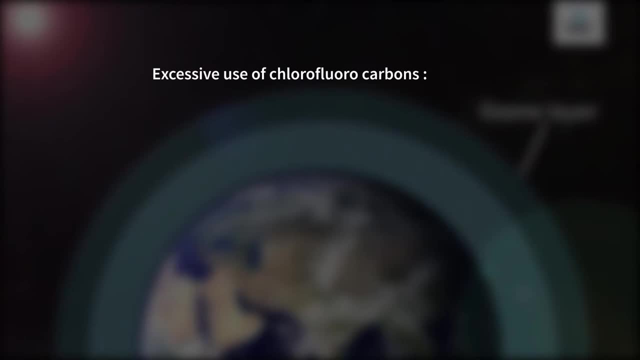 chlorofluorocarbons and their reaction. In here we see that chlorofluorocarbons are decomposed by the ultraviolet rays to highly reactive chlorine. Now this chlorine which is produced is in its atomic form, and we can also call it. 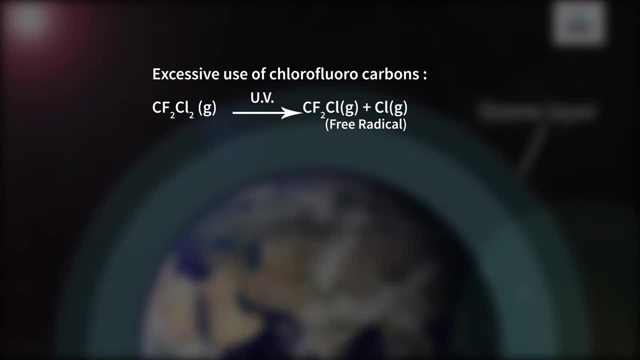 nascent chlorine. So this nascent chlorine, or the free radical chlorine, it reacts with ozone and it results in the formation of chlorine monoxide along with the oxygen molecule. Now this is the main reason for causing the depletion of ozone and this chlorine monoxide it further reacts with. 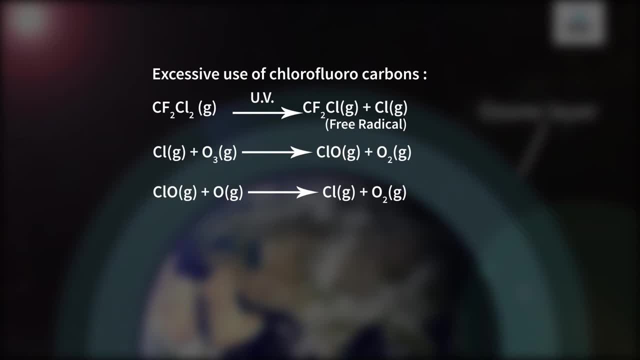 atomic oxygen to produce more free radicals of chlorine. So, as we see, more free radicals of chlorine means more reactivity. So here we will see that again. this free radical, it destroys ozone And this process it continues, giving rise to large scale of ozone.